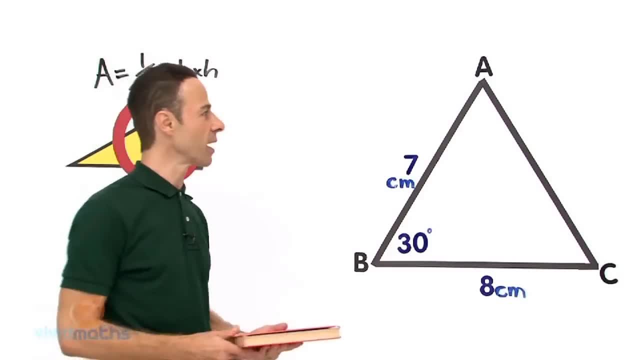 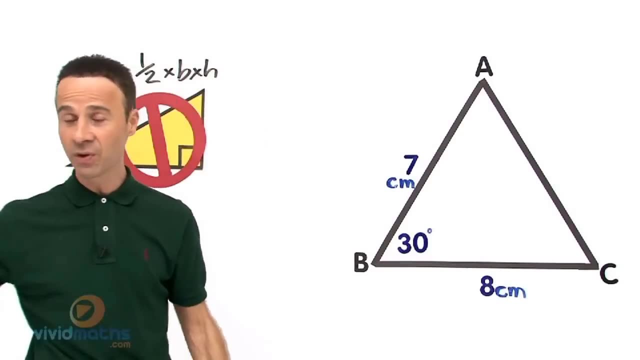 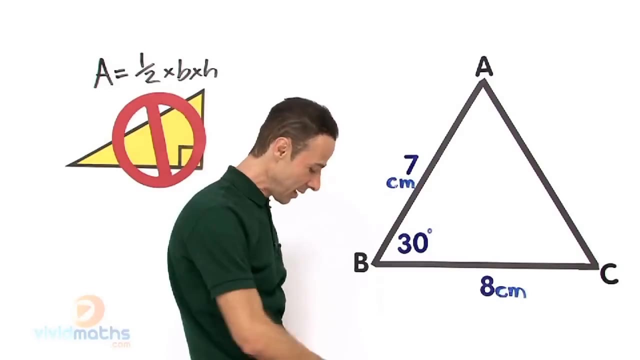 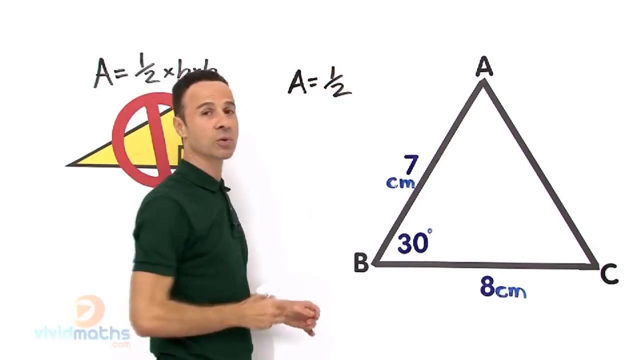 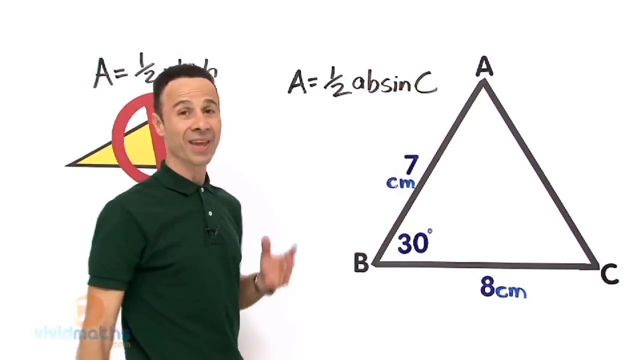 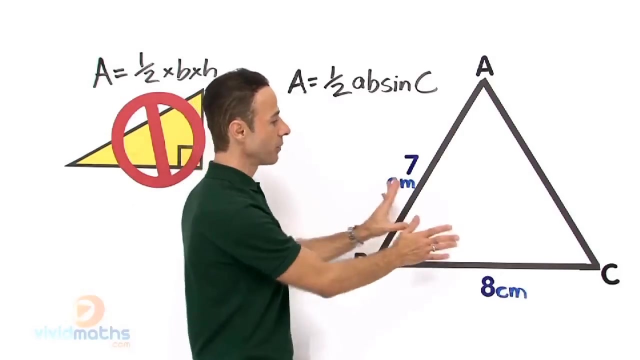 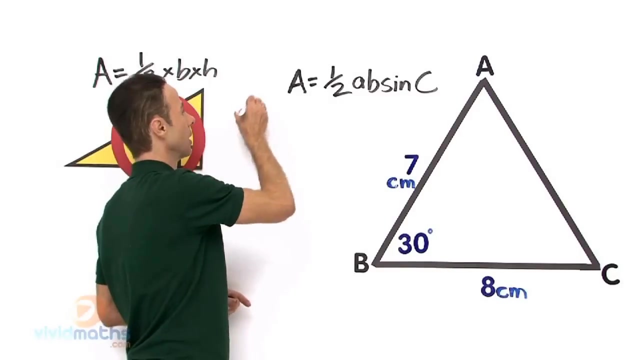 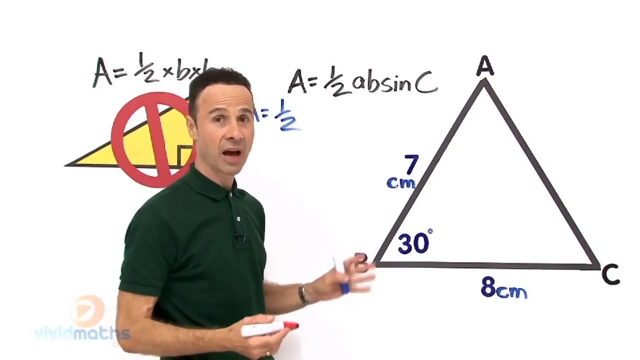 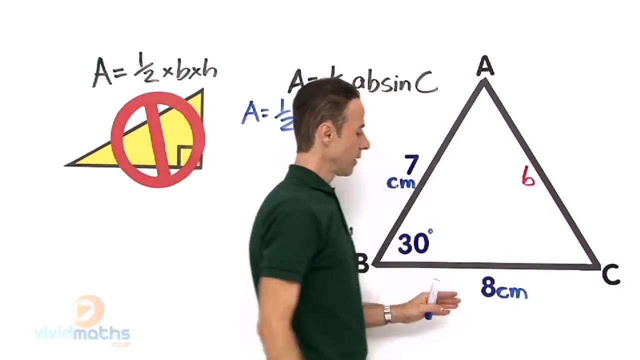 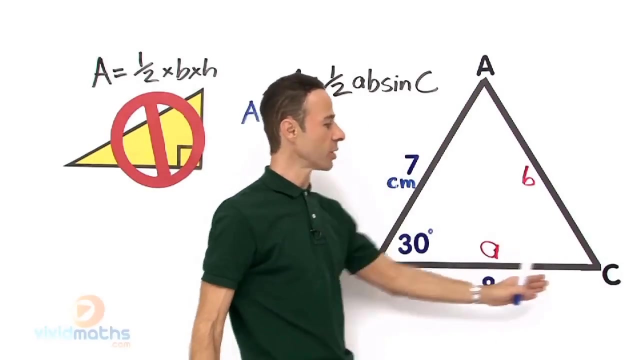 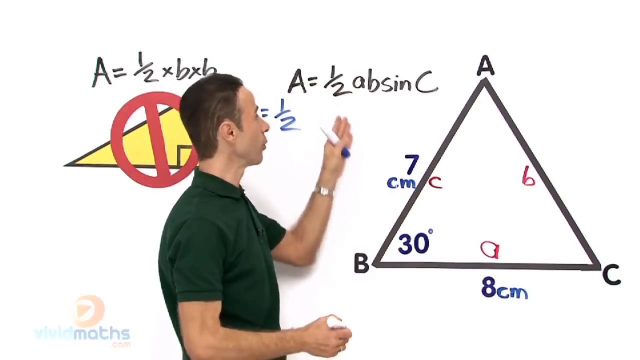 And I wonder if I can remember that new formula, it goes something like the area of a non-right angle triangle, non-right angle, here we are, non-right angle triangle area. I am going to give you that formula now. It is a fabulous formula, it is a new tool that we can use to find areas, we don't need that formula. It is area equals a half, that looks familiar, AB sine C. So if the angle we are given is C, then the two lengths in between is the angle we go for. In this particular instance, in this particular example, if I was to modify this formula that I just picked out of the book and modified it to suit this particular triangle, the formula would go something like this. It would go as A equals a half, now we got to put in the lengths here so that we can identify where they are because the lengths are opposite the capital letters. Remember what we did before? So if we got a capital B here, then little b is there. If we have a capital A there, which is the angle, then the length across here is little a and also if we got the angle there C, the opposite here the length is going to be little c. So there are all opposites and we were to put them in this triangle here, then we would have something like this. It 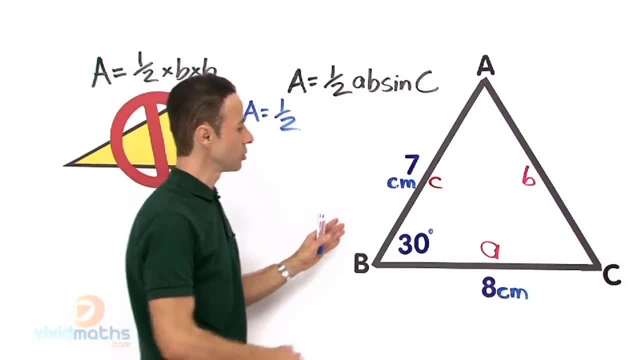 would be a half times, now the two ones on the side, they are the length of the triangle. 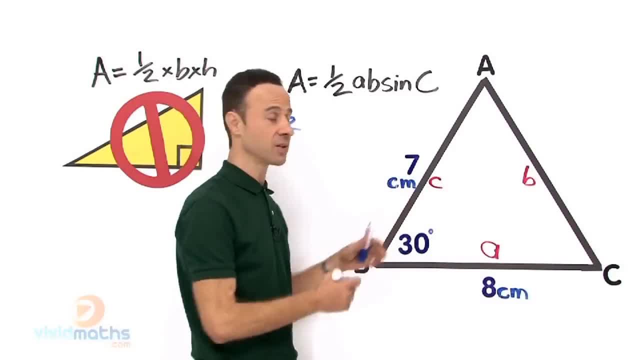 So we are going to put them in this triangle here and we are going to put them in this triangle here. side as you can see is the C and the A. So we will start with A and C so that will be 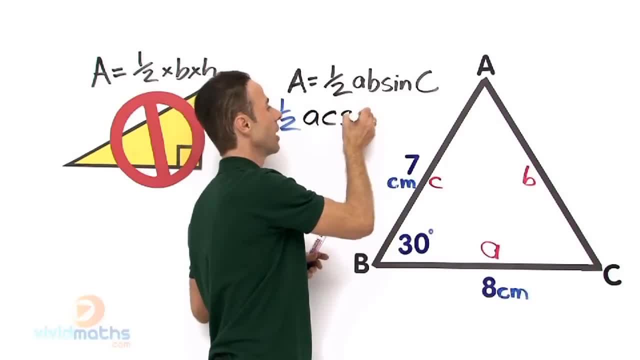 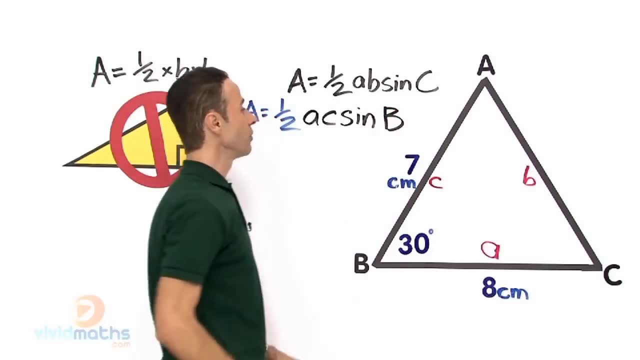 A times C times sine and the angle which is the capital right over here the angle see that that is B. So that is our new formula that is what we are going for. 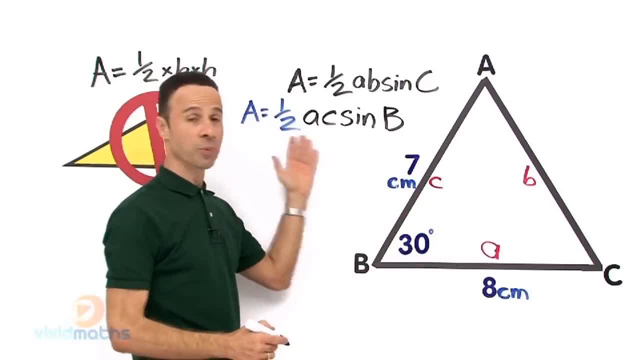 Ok so let us take the values from here substitute them in there and we will be able to work out the whole area of ABC triangle so let us do that. 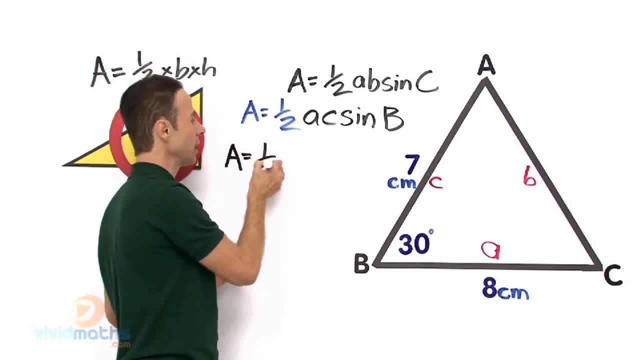 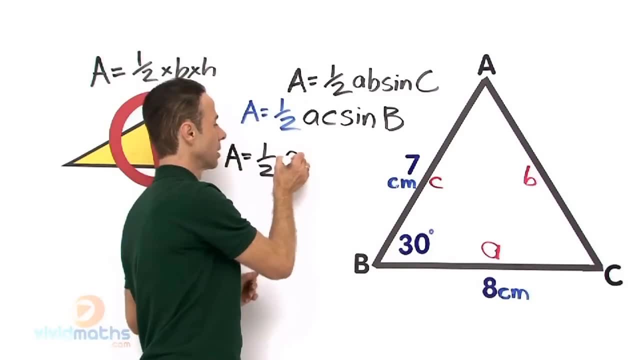 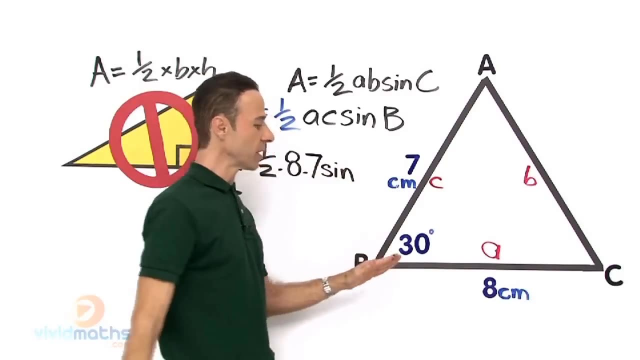 So the area would be A equals one half times AC here is a little A right there 8cm times little C which is 7 and then we finish off with sine the angle that we are given right